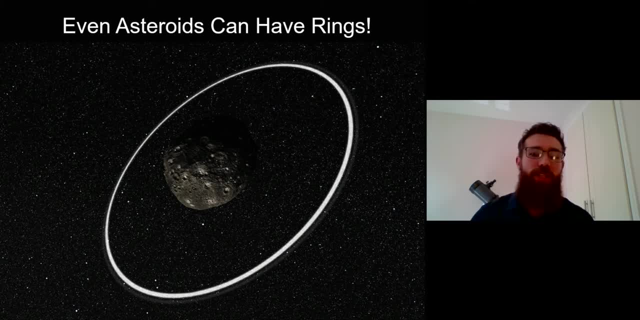 that have been discovered that are thought to have these small ring systems around them towards the outer part of the solar system, which is quite an interesting idea. So it's not just going to be just confined planets. Smaller objects can potentially have planetary rings. So what is? 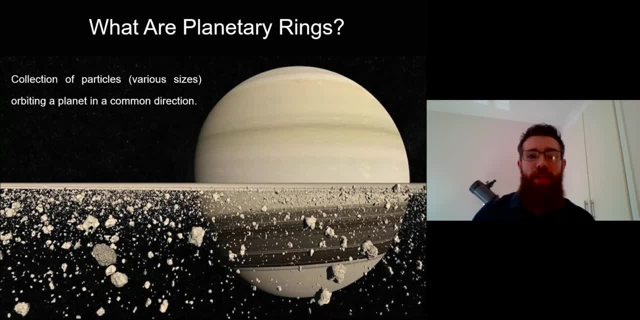 a planetary ring. Well, it's basically just a collection of particles that are orbiting in a common direction around the planet. So on the previous slide you saw an asteroid, So maybe that's a not a planetary ring. It could be an asteroid ring or something similar, But a. planetary ring is just a collection of small particles. Think of a small asteroid ring. for the time being. That's something similar. It's a collection of small particles, But that's not exactly the same thing as a planetary ring. You can see that on a planetary ring it will be a. 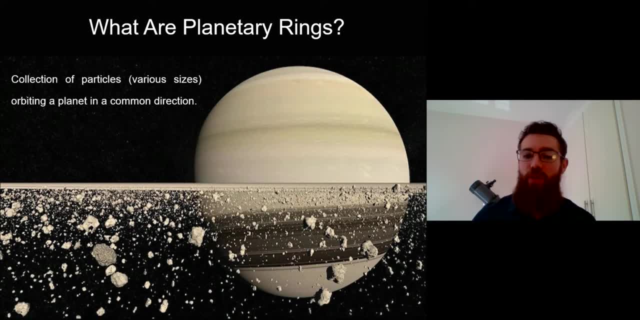 ring of some other thing as well, But a planetary ring is just a collection of small particles. Think of them as very small moons. They're all moving mostly independently and they're orbiting in a common direction, around a planet. So that is what a planetary ring is. 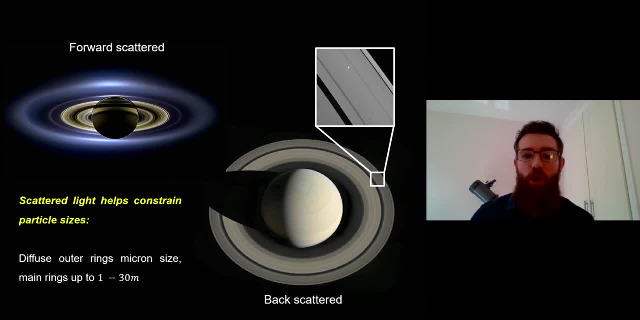 Now you saw on the last slide. you know the particles there. The rings are made up of a variety of different sizes of particles. you know from all the way up to the size of a house, down to kind of micron size. So very, very small particles. But how do we know that We can't just 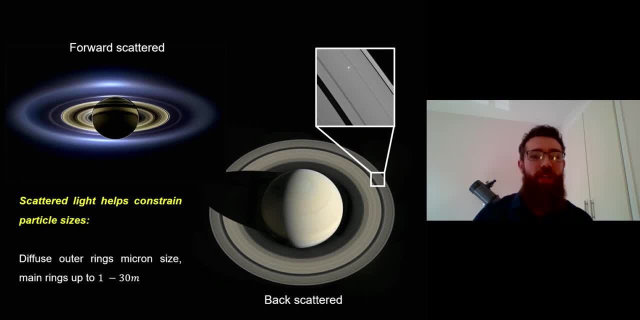 go and measure them with a ruler. So one way we can actually work out the size of these particles is by looking at the way that the light is scattered off these ring systems. So again, taking Saturn as an example, on the top you've got forward scattered light. 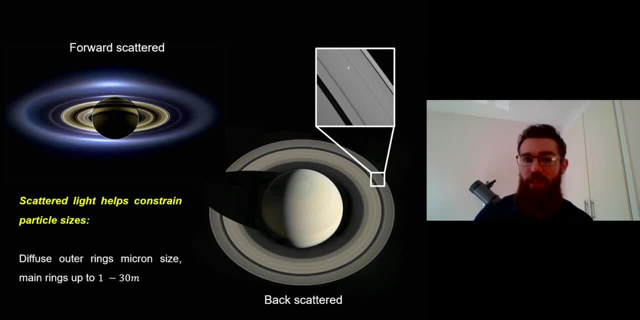 And we can work out the smaller particles from forward scattered light And at the bottom you've got back scattered. So what does that actually mean? Well, forward scattered is where the Sun is actually behind Saturn And the spacecraft that's taken that image, which would have been Cassini. 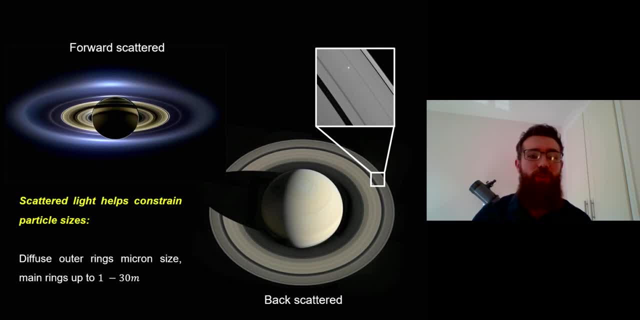 is kind of where we're looking at, So out of the actual screen, And what happens there is: the light is passing through the rings and it's being scattered forward so that we can see it. It's the same effect that you would have if you were driving down the road on a sunny day. 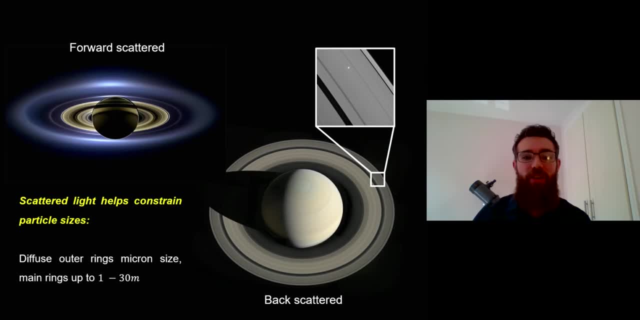 and your windscreen is basically scattering all that light into your eyes. You've got very small fine particles on the windscreen which are the light that's being scattered through the rings, And it's the same effect that you would have if you're driving down the road on a sunny day. 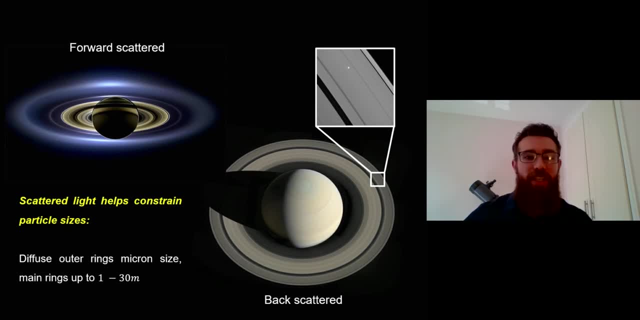 It's causing that forward scattering, So the smaller particles typically forward scatter more than the larger particles. But you can see these outer rings are visible in this particular configuration. Now, normally from Earth we can only see the back scattered view of Saturn or the 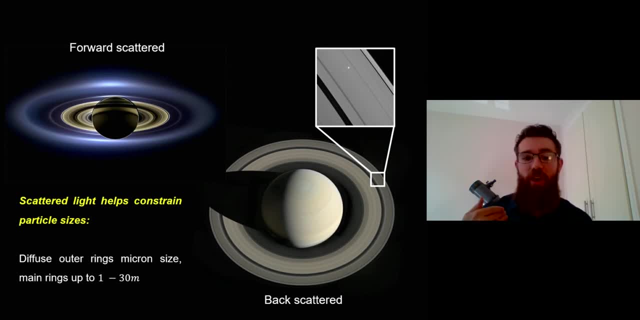 rings, which is down on the bottom right, And that is just the light that has been reflected back off the ring system back towards where the light source is, And larger particles are going to typically reflect this light or backscatter this light. So, looking at the way the light is, 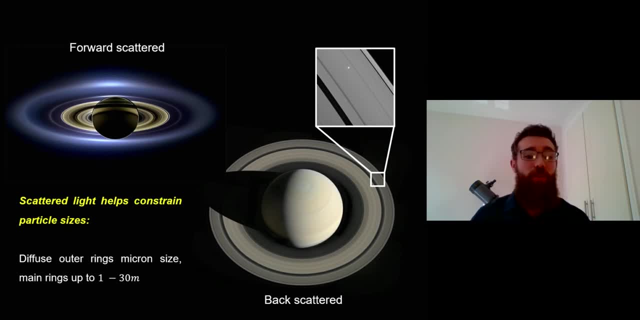 scattered off the rings, we get an idea for the size of the particles, And from doing so you know they're on the order of metre size at the largest and down to micron size. You can also work out how thick the rings are, their optical thickness, by 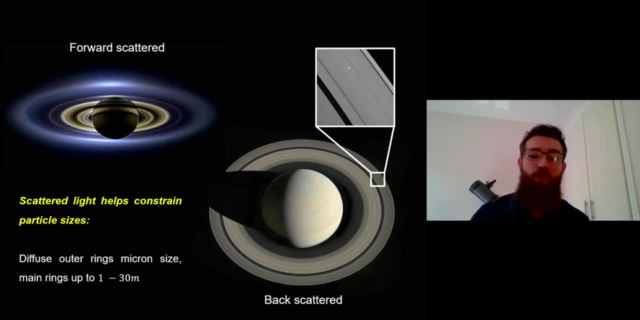 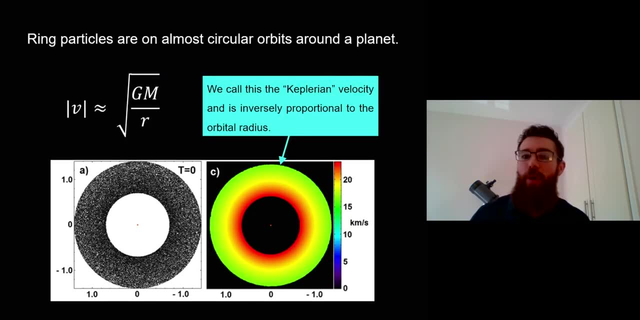 watching a star, pass behind it because you can measure the brightness of that star, which is shown in the white box. So one of the key things about planetary rings, then, is that they're generally quite circular, So they're not very elliptical, I mean. 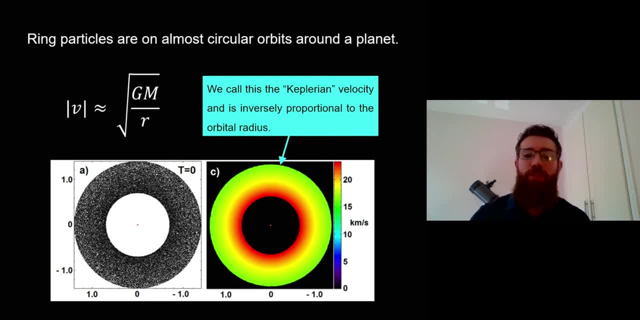 if you look at the finer scale structure of Saturn, there is some kind of change to that, But as a general rule they're going to be on a fairly circular orbit. Now, if you know your Keplerian laws, where we call this velocity, these ring particles have as they're on their orbit. 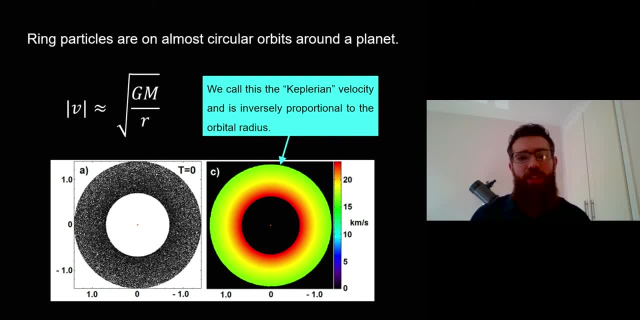 like a Keplerian velocity, And what it means is that the closer to the planet they are, the faster they're going to orbit In order for them to have that circular, stable orbit. So if you want to work out what those velocities might be, you've got a very simple equation there. 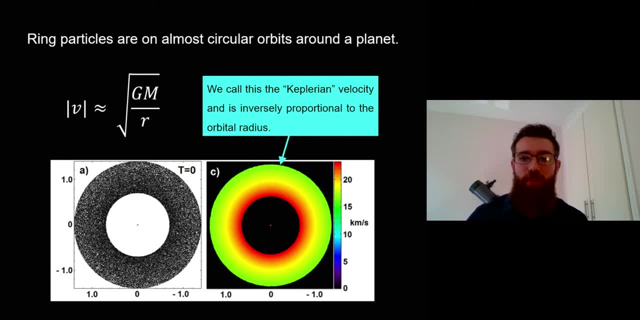 at the top. But just to give you a visual example of that, for some simulations I've done in the past, I've got a ring system, just like Saturn there, of all these particles orbiting around it And then the right hand side. you've got a colour image of the velocity of the particles as they're. 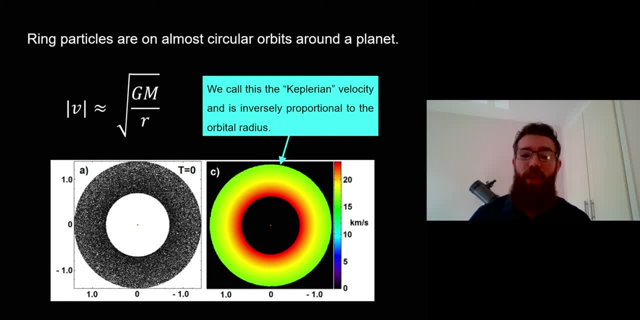 on their orbit And you can see that the closer they are to the planet, the faster they orbit. And we call it a Keplerian velocity. But also, if you think about all those particles together, it's also kind of a Keplerian shear, shearing flow. So the closer particles are orbiting faster. 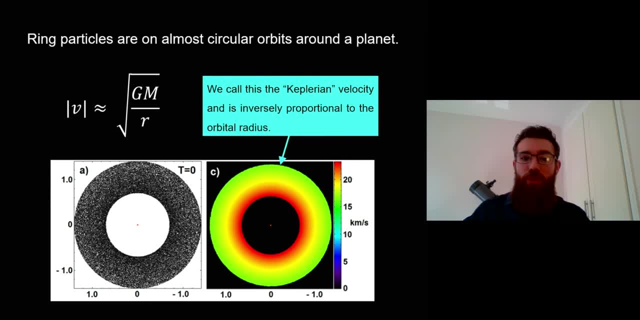 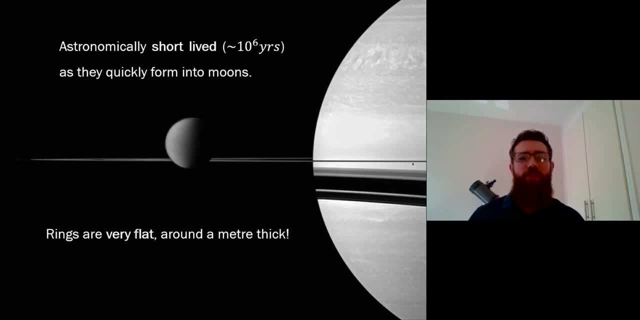 than the ones outside, So it causes this kind of shearing motion, which actually gives a lot of the structure we see in Saturn's ring. Now, something else that's quite curious about these planetary rings- specifically with Saturn as well- is they're very, very thin, So they're actually only on the all. 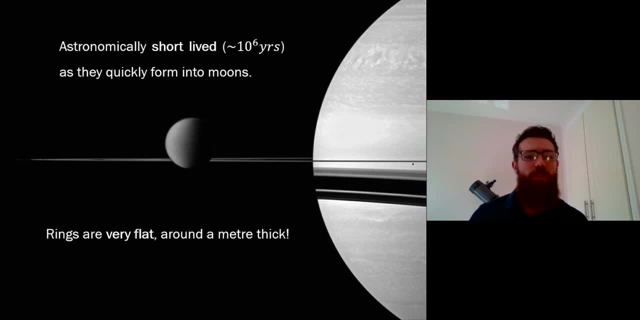 or the order of a metre thick, which means that they're almost just one layer of particles. You remember, in the size of the particles they're on the order of that metre size, the biggest ones. So the rings are only a metre thick. There's only really one layer of particles. 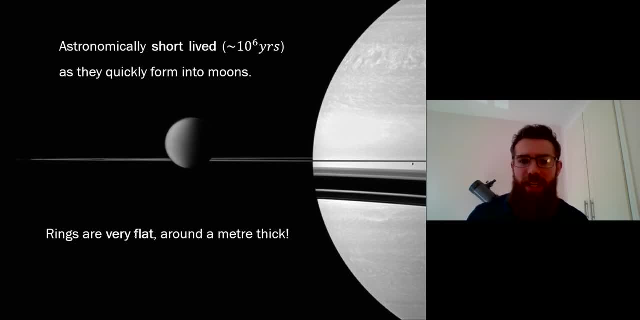 there in some places And also they don't particularly last very long. They very quickly will form into moons. So over time the edge of the ring system will kind of clump into a moon and then it will kind of move away And this is what's formed a lot of our 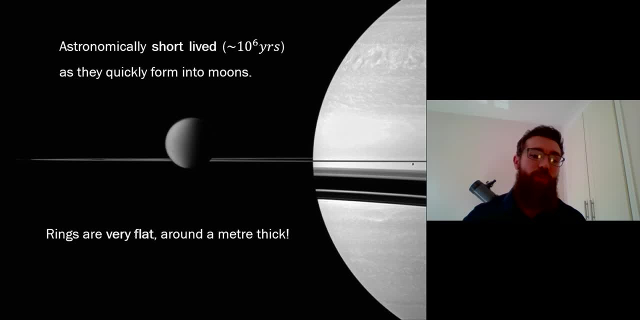 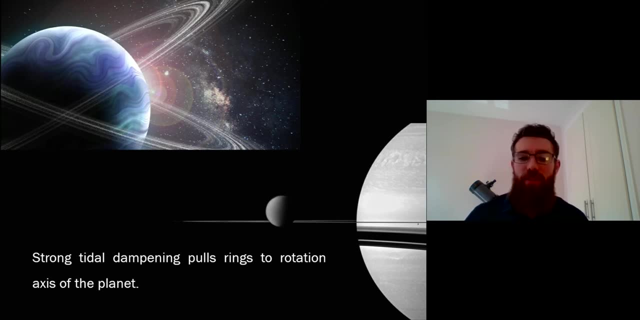 moons around Jupiter, Saturn and all the other planets. really, These rings will very quickly form into moons. They generally match the rotation of the planet, So they're kind of aligned to the rotation axis along the equator. Now I've got a nice image at the top there. 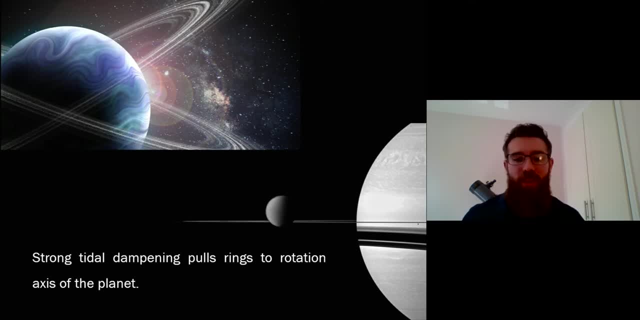 which shows you a couple of planetary rings around a planet which is obviously an artistic impression And realistically that's not really going to be that possible because it will very quickly relax down to the rotation of the planet And the reason for that really is that the planets are not spherical, They're not a perfect sphere. They're kind of bulging at the equator a little bit, which means that there's more mass there. But gravitationally, as the rings are orbiting around, there's a difference in the gravitational force And it very quickly basically dampens that movement or that inclination. 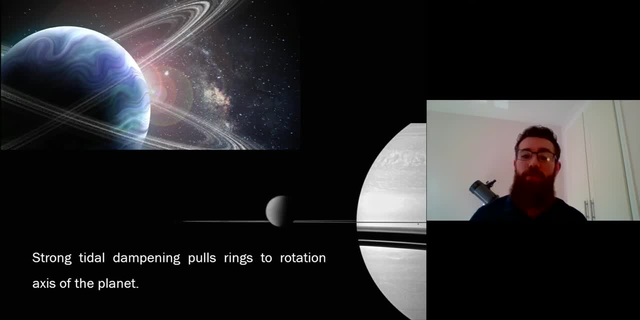 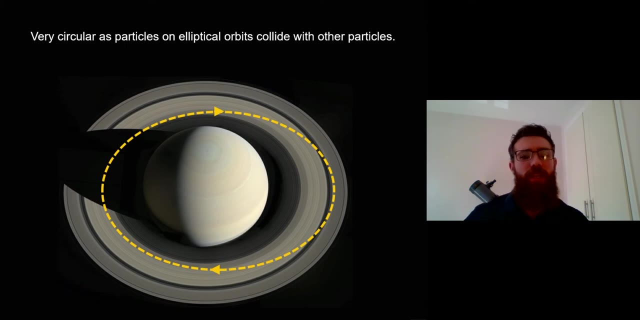 so it matches the equator of the planet. So even if it did form inclined, it's very quickly going to be pulled to that rotation of the planet. The reason why they're generally quite circular is that if you had a single particle, so remember, all of these particles in the rings are orbiting. 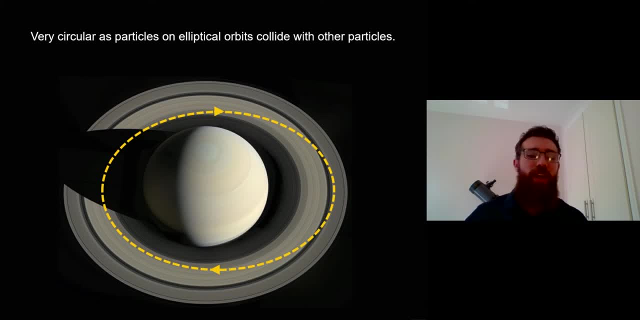 kind of on their own. They're like very small moons And if they're on an elliptical orbit they're going to pass into the path of other particles. They will likely have a collision And that movement into the path of others and the collisions they then have. 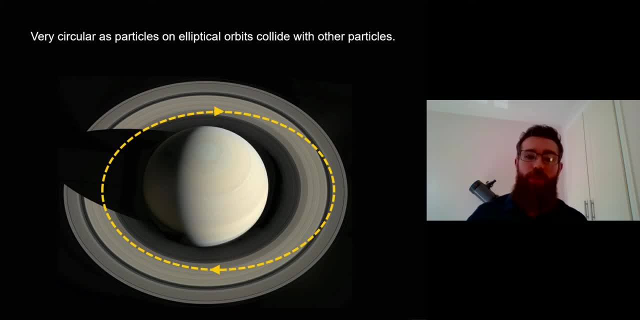 stops that kind of outward and inward movement. So if they're on an elliptical orbit they actually move away from the planet and towards the planet as they go around, But as they do so they'll collide with other particles, So it dampens down.